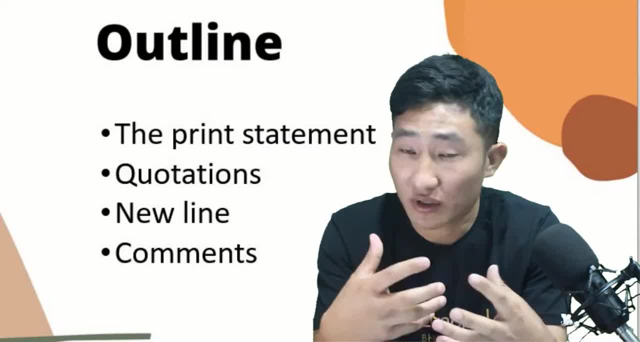 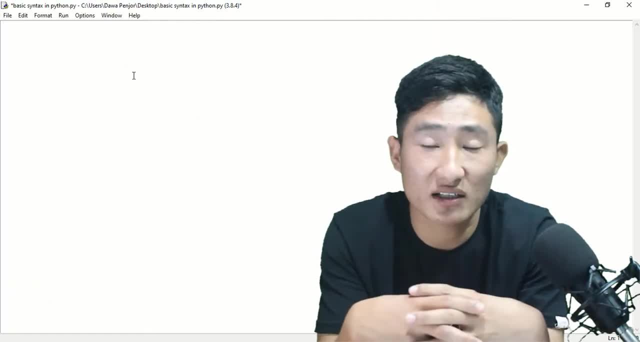 basically, I'll be talking about the print statement and the use of quotations, the use of new line and including our commands in your program for this lesson, for all the Python series lesson- I'll be using a Python text editor, so if you haven't installed Python text editor, I would 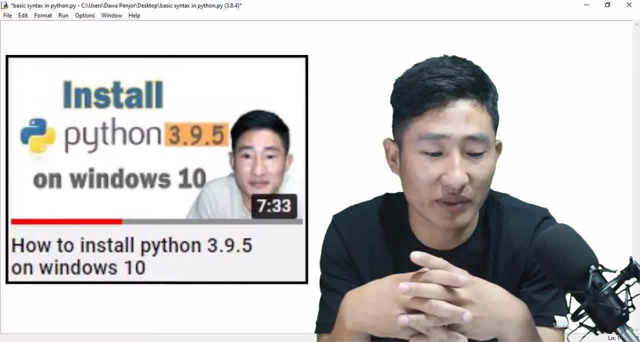 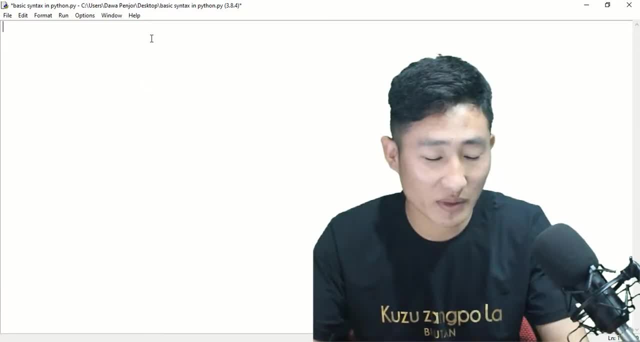 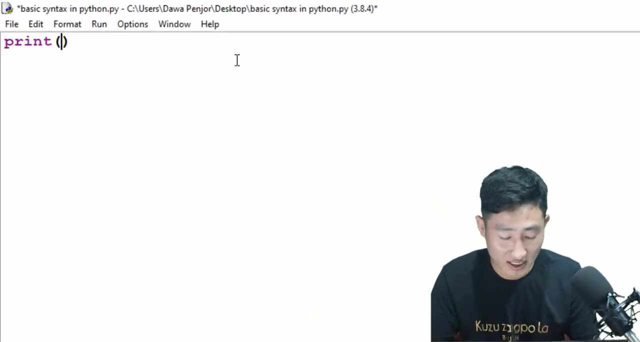 recommend you to watch my video on how to install Python and Python ideally so I'll be using this text editor till the end of my Python series. now I'm here in my Python, ideally the basic syntax to print any output. so first thing is you should write a print and then here you can. 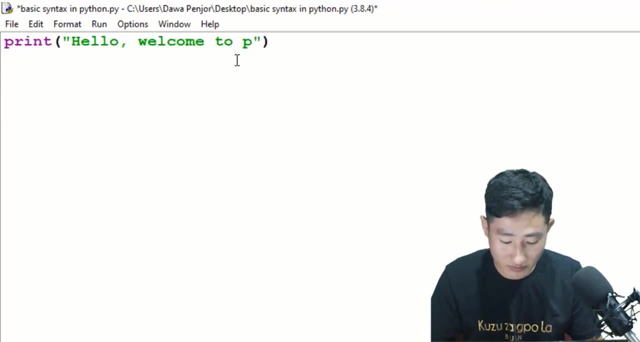 pause any string. so hello, welcome to Python programming. let's say this one is my first Python program. so this one is a print statement. I have used the print here. it will print the output in the console window. so anything that you want to see on output window, then you should include everything inside the print function. if I run this program, so you. 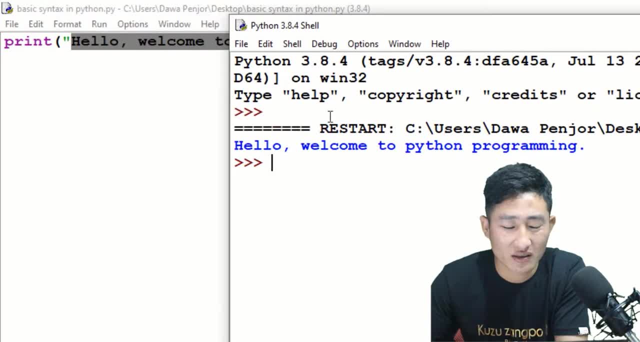 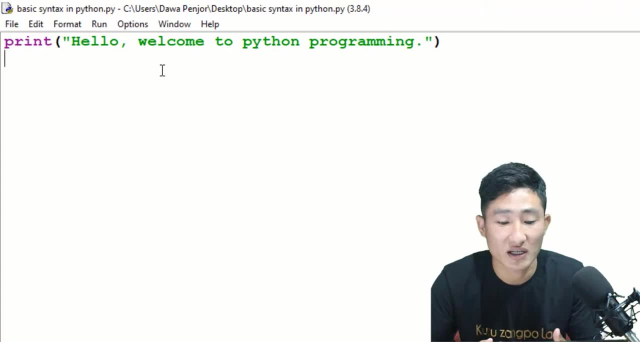 should. you should see that. hello welcome to Python programming. this is the main functions of the print print keyword. the print function is used to print an output on the console window. you might be wondering that you see that it. it was enclosed inside a quotation mark. this is because anything that 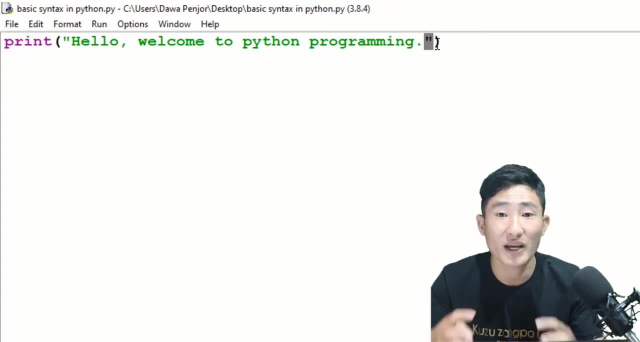 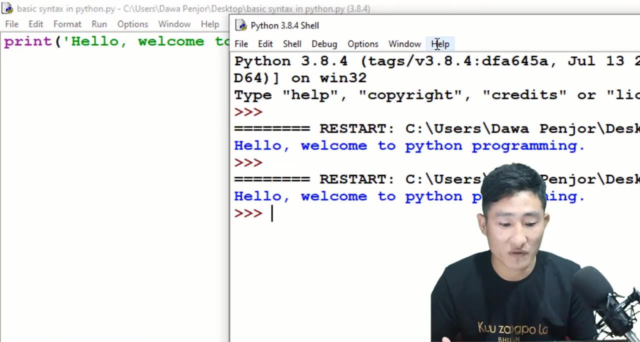 any. any text that you want to print on our output console, it should be enclosed inside the quotation mark. but if I replace this with a single code, okay, if I run this program it works perfectly fine. you see that? hello, welcome to Python programming. we see the same output. 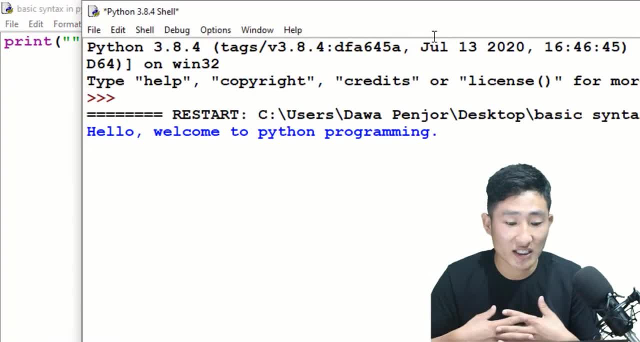 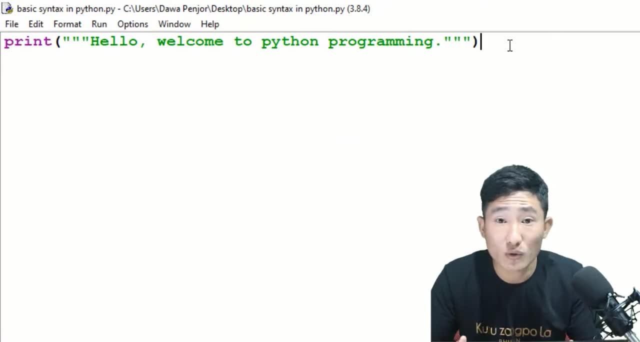 okay, even if I use triple code and run this program, you should see the same output. so basically, what I'm trying to explain here is in a print function, like whether you use a single code, code, double quote or triple quote, it conveys the same meaning and you should see the same output. 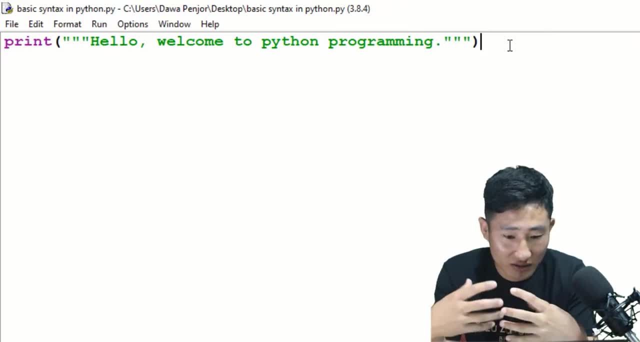 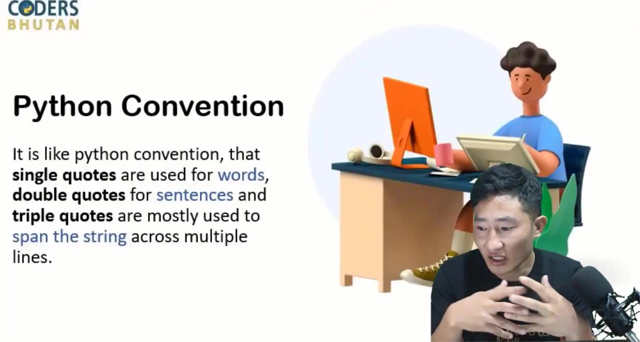 but, uh, under certain circumstances, uh, single quote, double quote or triple quote, there are certain restrictions or, most appropriately, i would say that there is a python convention. single quotes are used for words and double quotes are usually used to print the sentences, and triple quotes are mostly used to print a multi-line statements in the python. so, for example, 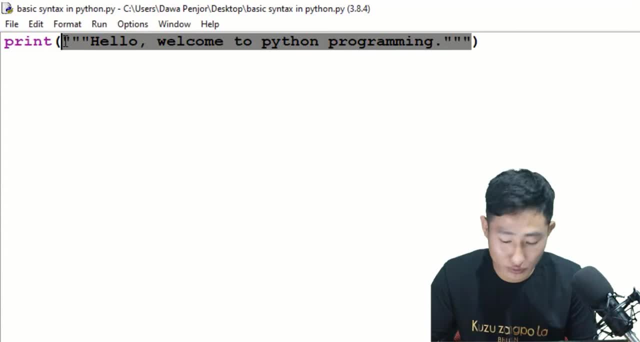 let's say now: uh, i'm using, i want to use a single quote here, and then i want to print something like this: it's: uh, okay, so i want to print something like this: now it's rainy day and i have enclosed inside a single quote. you see that in earlier program it works perfectly fine, but in in this, 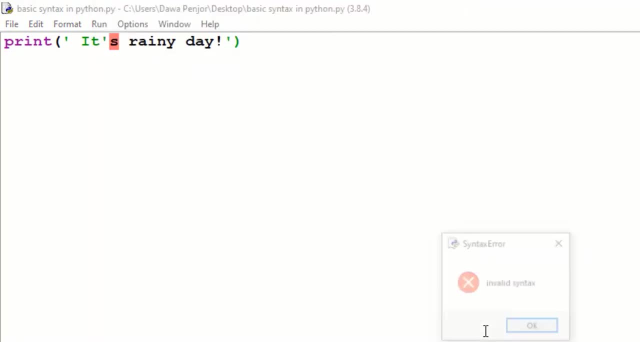 case. now, if i run this program, you should see that it does not work. we get an error in valid syntax. this is because sometimes the use of single quote or double quote or triple quote makes difference. so this is because we have. we have started with a single quote and now the single quotes gets end. 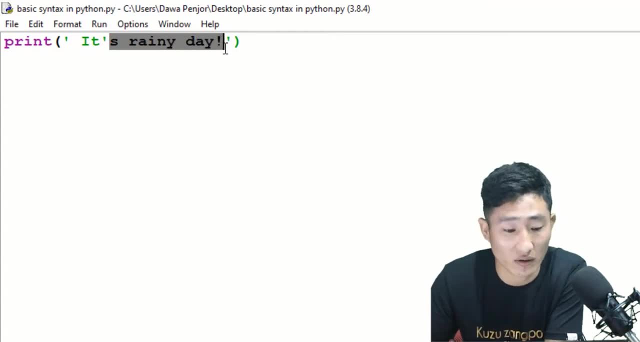 here and the rest of the line of the text will be error, so that's why it does not work. in such cases, you should use a double quote. okay, maybe a double quote, and then, if i run this program, you should see an output. it's rainy day. what i'm trying to explain here is the use of single quote. 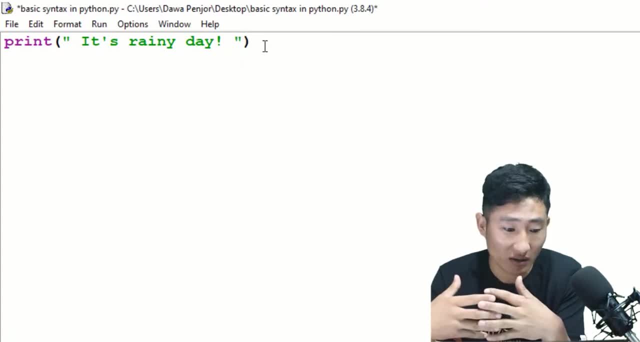 double quote or triple quote differs from, like, the text that you are including inside a print statement. so now let me talk about uh, triple quote. now inside a triple quote and run the program. you should see the same output. it's rainy day, but what is the advantage of using a triple quote? 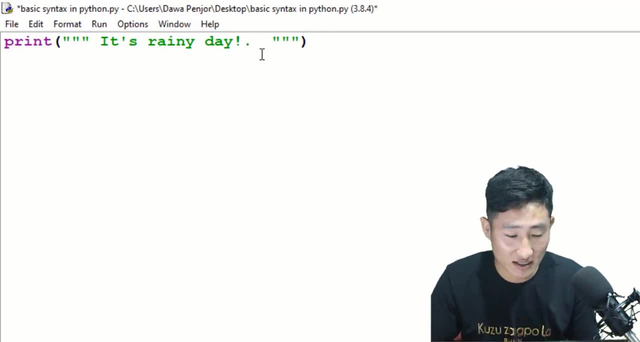 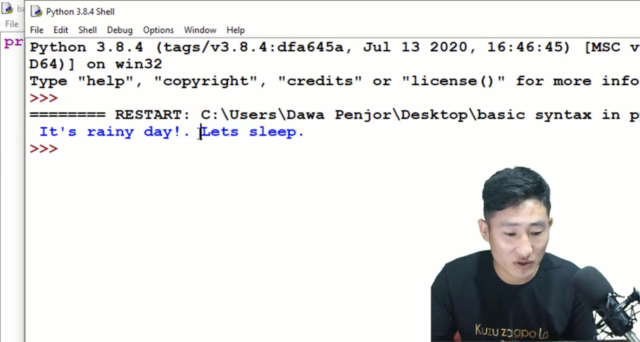 so now i want to increase, uh, the length of my sentence. so, it's rainy day? okay, let's select. okay, i want to print something like this: if i run this program, you see that, uh, you get the same output. but in such cases like it's rainy day and let's sleep, i want to put this output into a. 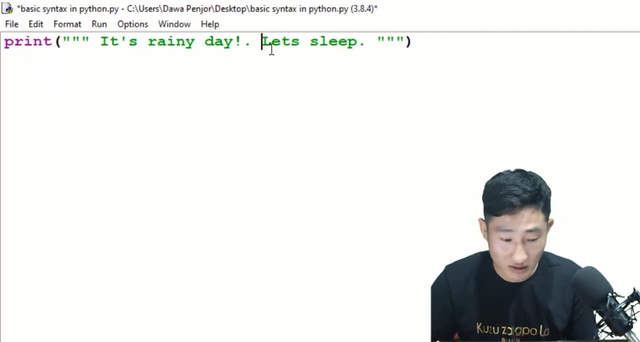 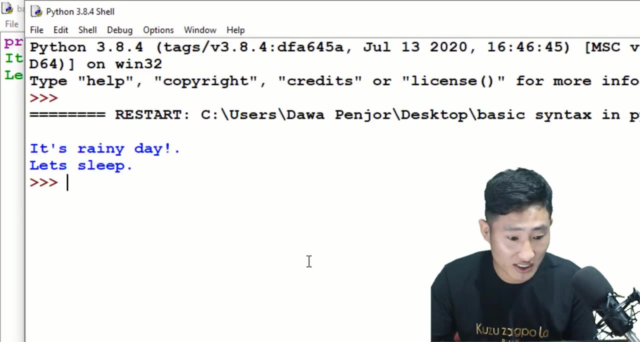 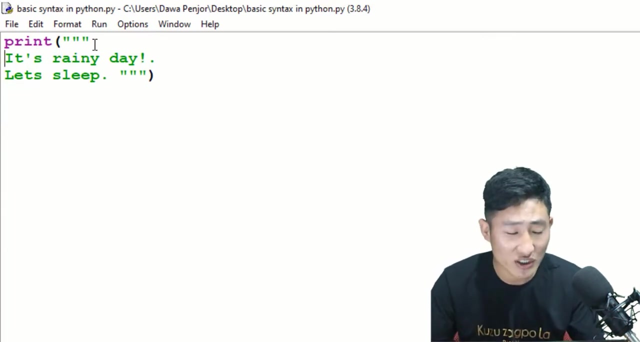 next sentence. in such cases, using like a use of triple quotes becomes very handy. if i run this program, you should see that it's rainy day and let's sleep. this is because the advantage is using this triple code is it is usually used to span the string into a multi-line. that means we 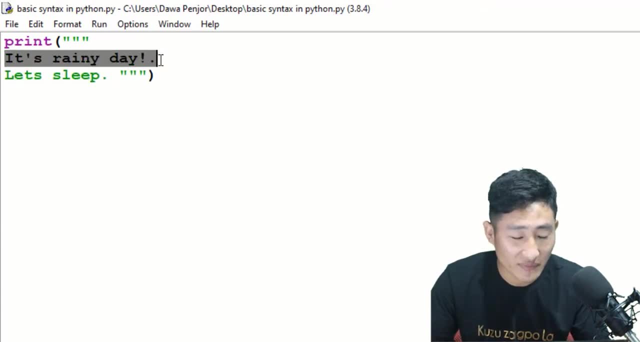 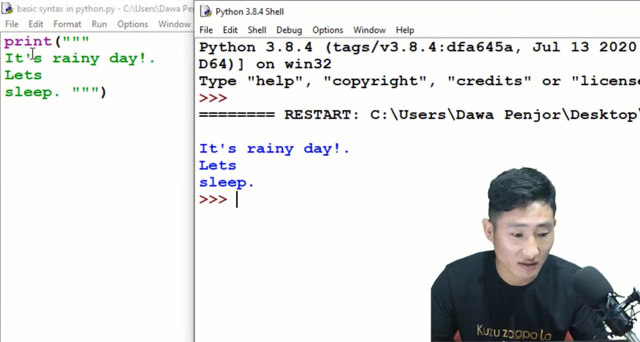 are like we are putting everything in the next line. so again, if i, if i put this late, slip in next line and run this program, you should see the same thing. you should see a triple quote again, if you like how I had been included in my text editor. see that it's a rainy day late. 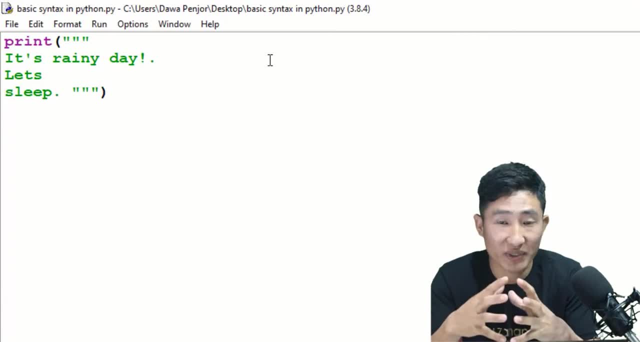 sleep. this is how a quotation works in the print statement. now let me enclose these with, like a double quote, and if I run this program, you should get an error. this is because it does not work to print a multi, multiple line of text. you should always use a triple quote. okay, but there is also another way of. 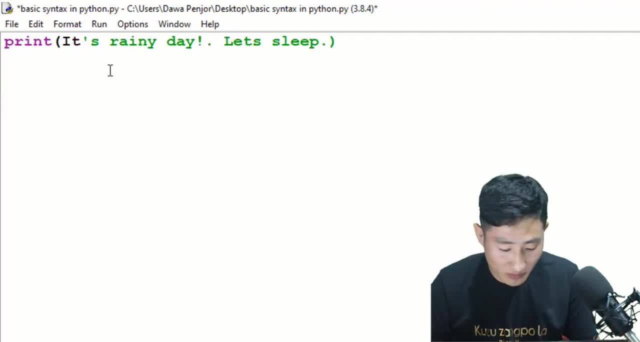 printing our text in a new line. let me talk about the use of new line. so new line is used to break the statements or print the text in a new line, so that the syntax to use a new line is: if I want to print, it's rainy day and let's sleep in. 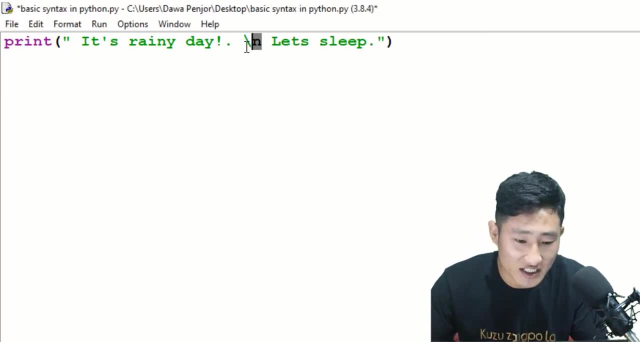 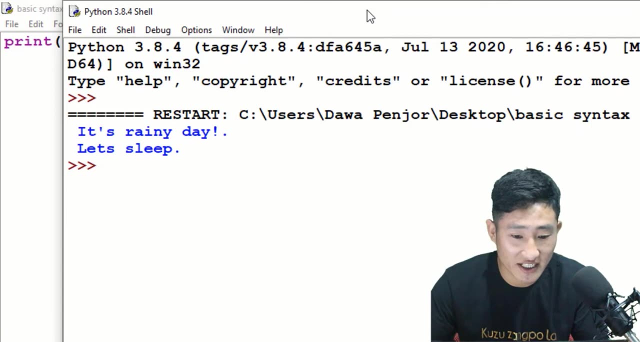 the next line. then you just need to put slash n. this slash n is for the new line. that means this let's sleep will be printed on a next line. so if I run this program, you should see that it's the rainy day and let's sleep. on a on the 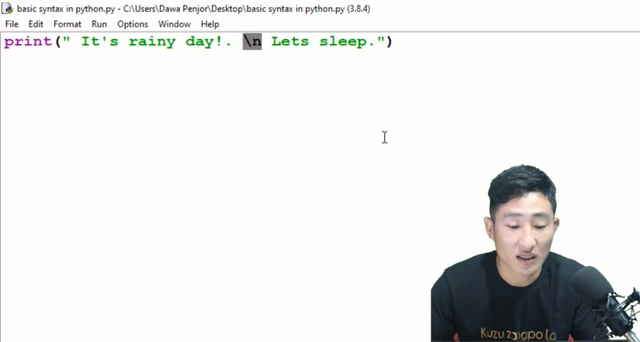 next line. this is because, before let's sleep, I have used a new line. these new lines are used to put the text in a new line, next line or in a new line. so now let me talk about the commands. so the commands always starts with the hash sign and then you can always print. 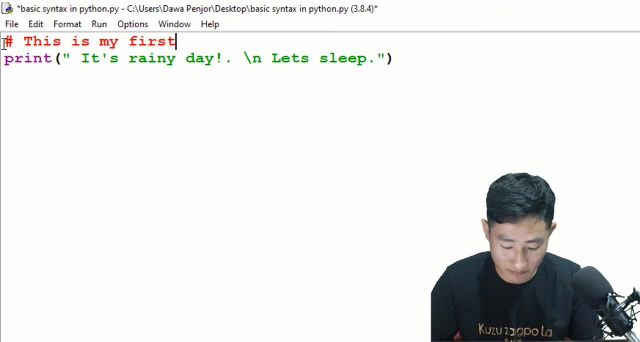 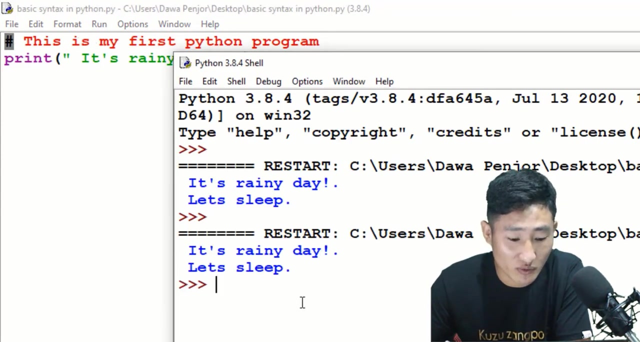 something like this: this is my first key Python program. this is my first Python program. now, this is a command, because we have started with the hash sign and if I run this program, you won't see- this is my first Python program. you will. instead, we see the text. that is, that has been. 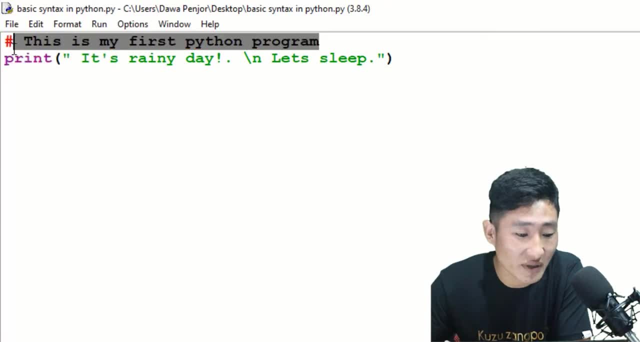 passed inside a print statement. this is because this command, like avoid it by the Python interpreter command, won't be interpreted by the Python and it is purely for, like a programmers, to explain about the block of code. so there are also other varies ways of including a command, so you can also include this. 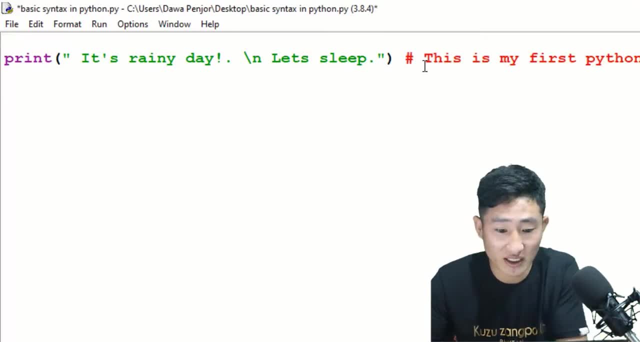 command somewhere here. now, if I put something like this now, the Python interpreter with interpret starting from here in it ends here and it won't interpret this because of this block of code. this line of code start with hash and anything that starts with the hash will be taken as a. 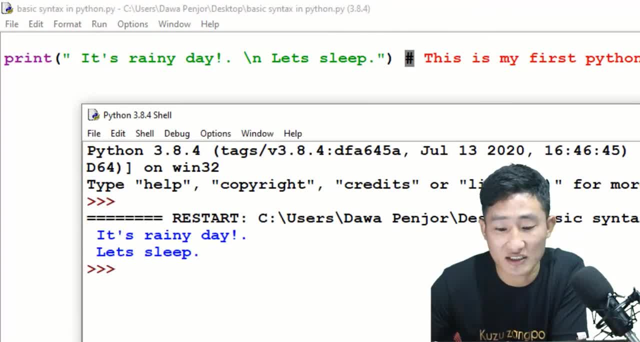 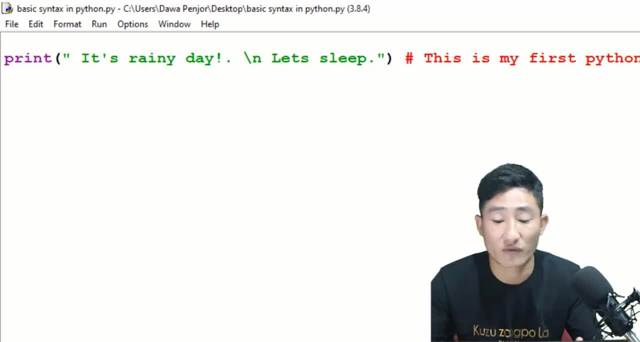 command. so if i run this program, you don't see this. this is my first python program or there is. there is also no any error. this is because this one is a command and it's for the like, for the programmers, to explain about the block of code. there are so many things that you need to know.